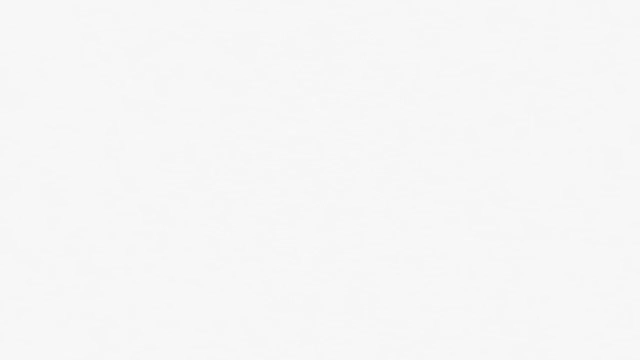 the rotation matrix and the displacement vector, And so it's important to first do the other method and make sure that you understand the meaning. Let's take a look at the origin of each part of the homogeneous transformation matrix before you start taking the shortcut method to the end. 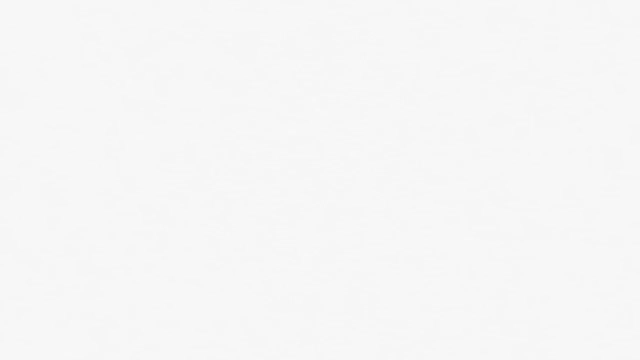 In this video we'll be learning this shorter Denevet-Hartenberg method to find the homogeneous transformation matrix. But keep in mind that the matrix that we end up with the end will be the same as the matrix that we find if we use the other method. 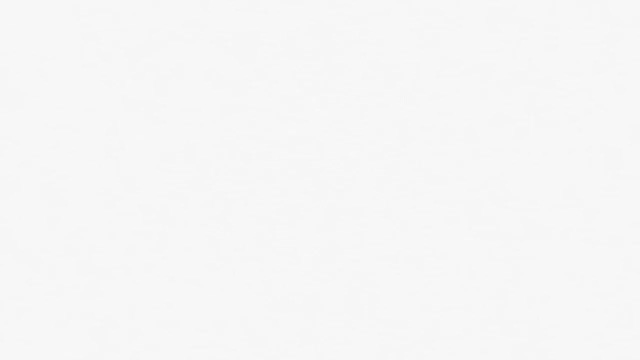 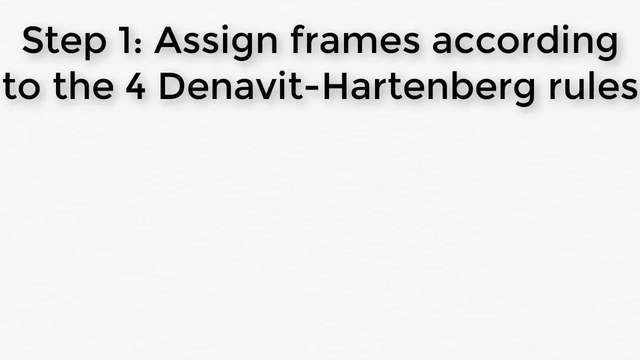 So, whichever method you prefer to use- you can use The Denevet-Hartenberg method- will find the sign for the transition matrix and then method proceeds like this. Step one is to draw the kinematic diagram and assign the frames. We have to make sure that we assign the frames according to the 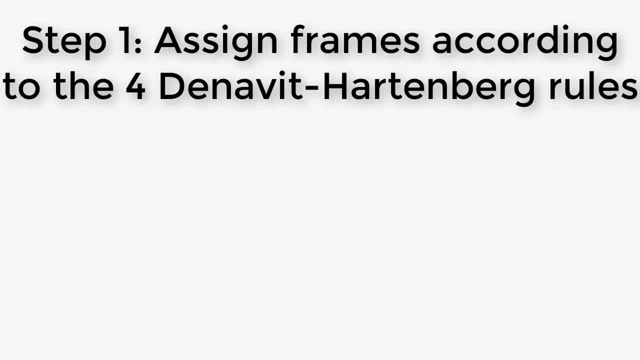 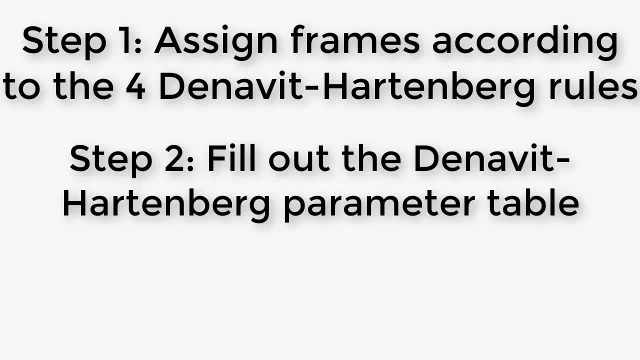 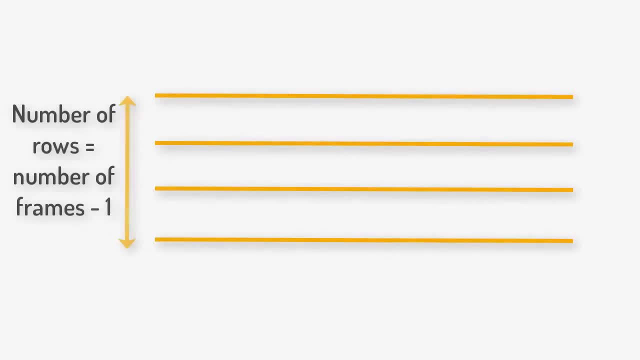 Denovit-Hartenberg rules. We already learned how to do this previously. Step two is to create a parameter table. To find out how many rows your parameter table should have, count up the number of frames in your kinematic diagram and subtract one. The number of columns in the table is always the same. We always. 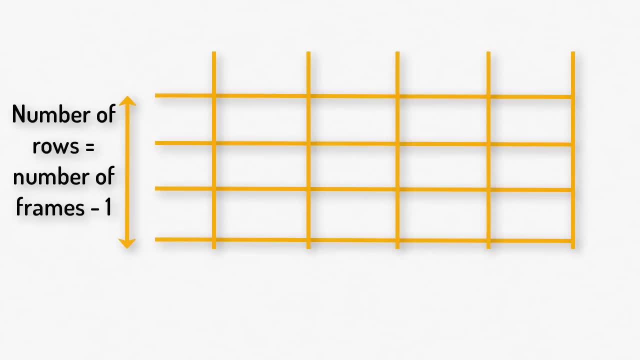 have four columns. Each column is for one of the four parameters. Two of the parameters in the Denovit-Hartenberg parameter table represent rotations, and the symbols that are used for these two parameters are unaligned alpha and theta. The other two parameters represent linear distances or 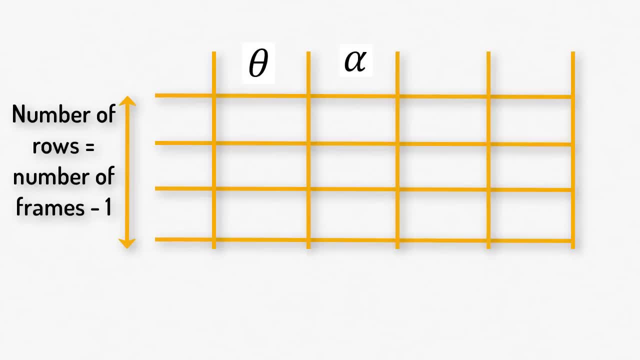 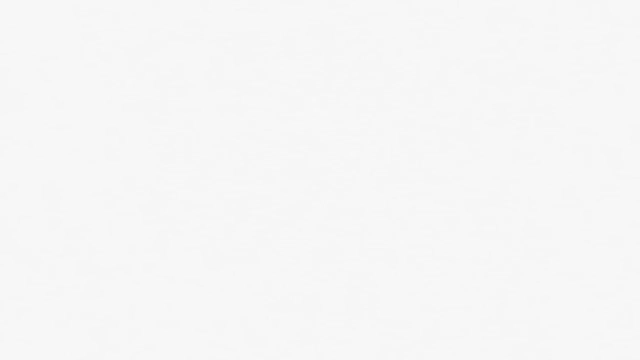 displacements. The symbols that we use for these two parameters are the letter R and the letter D. Let's take a look at the meaning of each of these parameters. To set up the explanation of the meaning of each of these parameters, I'm going to 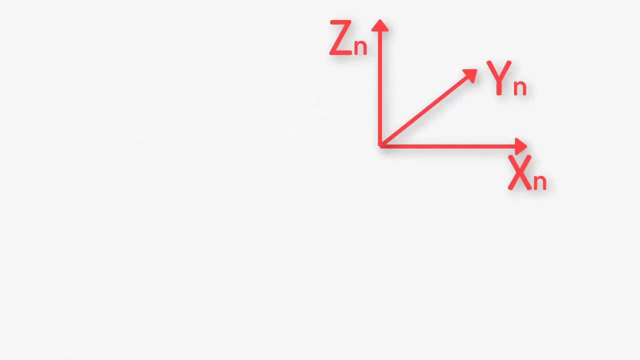 consider two frames. I'm going to call one of these frames frame n, and the other frame I'm going to call frame n minus 1.. So in a kinematic diagram, these two frames might refer to frame 2 and frame 1, or frame 1 and frame 0, or frame. 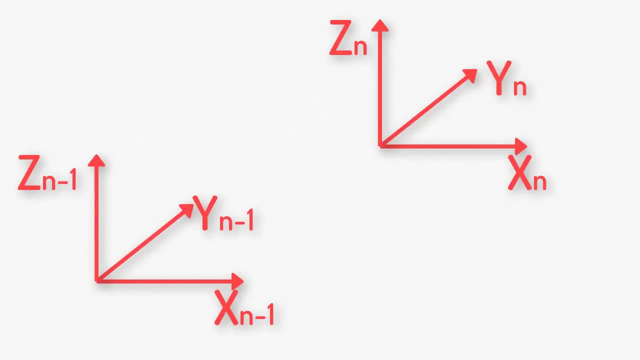 3 and frame 2.. n and n minus 1 could refer to any two frames that are next to each other. That's why I'm referring to them as n and n minus 1.. Let's start by looking at the parameter theta. Theta is defined as the rotation around z, n minus 1, that is. 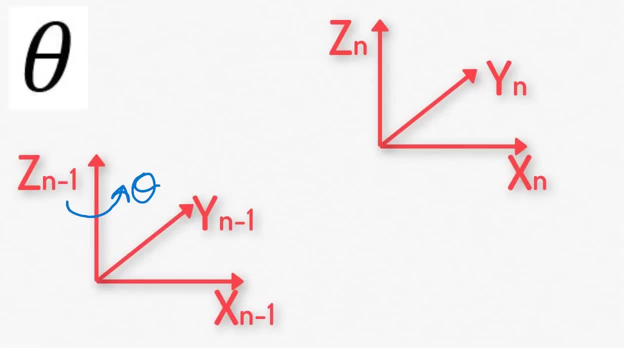 required to get axis x n minus 1.. To match axis x- n. keep in mind that this has to include also any theta rotation that is due to the joint. After I've defined each of these individual parameters, I'm going to give you a bunch. 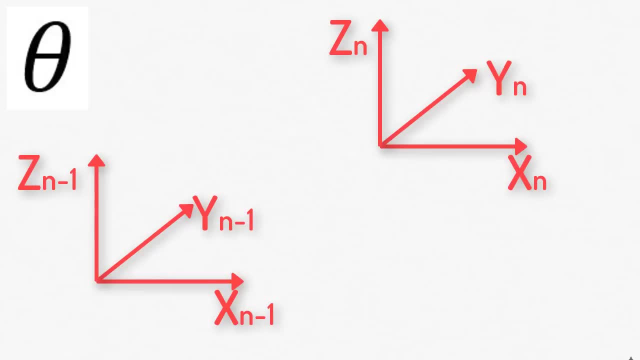 of examples, And these definitions will make more sense as we look at examples. So don't worry yet if you don't fully understand the definitions. I'm just going to start by laying out these definitions so that we can refer back to them later on. 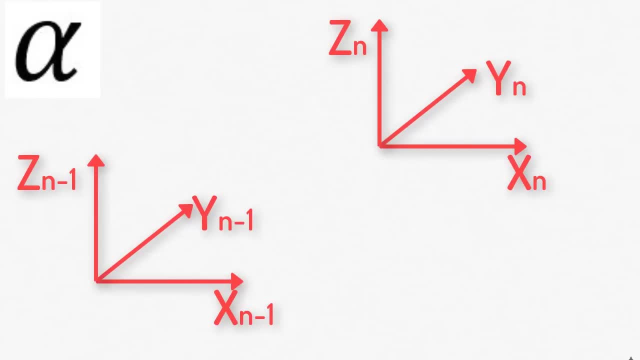 Okay. secondly, the rotation alpha is defined as the rotation around x n. that is required to get axis z n minus 1 to match axis z n. Now keep in mind that, even though the axis we're rotating around is the x n axis, the 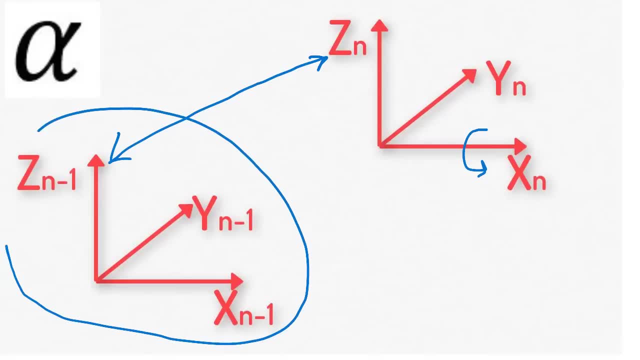 frame that we're going to rotate is the n minus 1 frame. In other words, we want to ask ourselves how do we have to rotate the n-1 frame around the axis x n in in order to get the axis z n minus 1 to match axis z n. 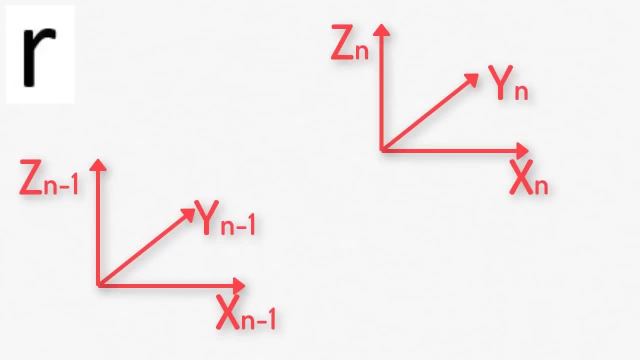 To find the parameter r, we look at the distance r from n minus 1 to n minus 1.. the center of the n-frame, The r-parameter, is defined as this distance along the xn-direction. So I'll extend the xn-axis and we'll look at the distance between the centers of these. 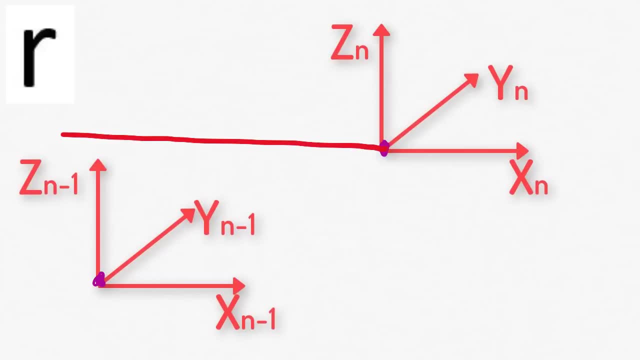 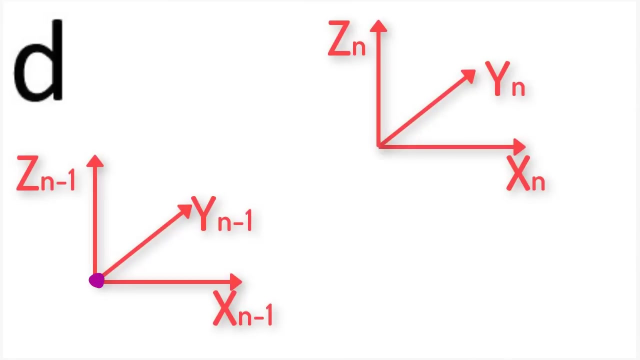 two frames, only in the xn-direction. This is the parameter r. d is the other linear distance parameter. It's defined as the distance from the center of frame n-1 to the center of frame n, measured only in the zn-1 direction. 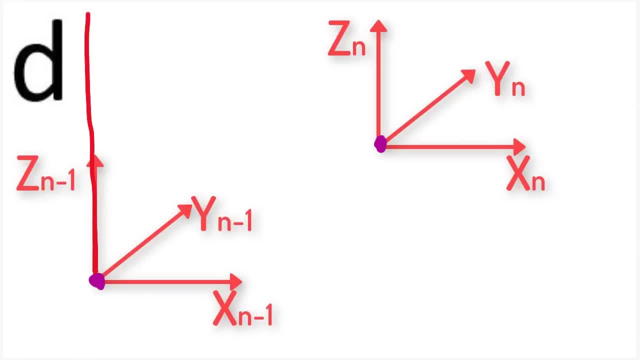 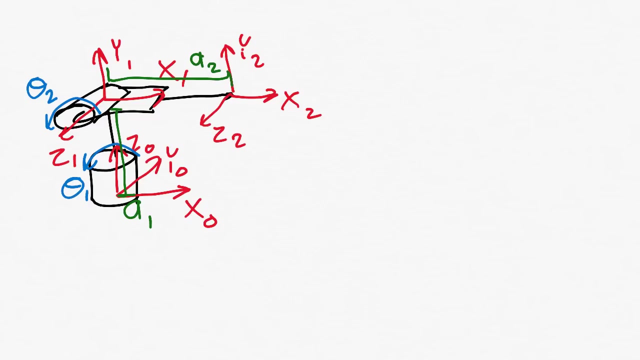 So I'm going to extend the zn-1 axis and then the d-parameter is defined as this distance. right there, Okay, let's look at some examples and see if we can better understand the meaning of each of these parameters. Here I'm showing the kinematic diagram of a two 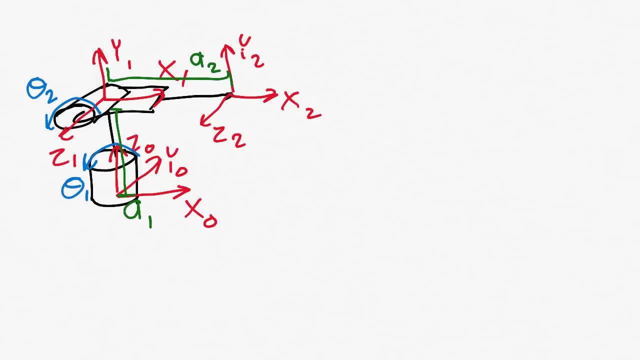 degree of freedom manipulator that is oriented according to the articulated manipulator. So it's not a full articulated manipulator, but I've started with the articulated manipulator and I've sorted it out as if we're going to be drawing an articulated manipulator. 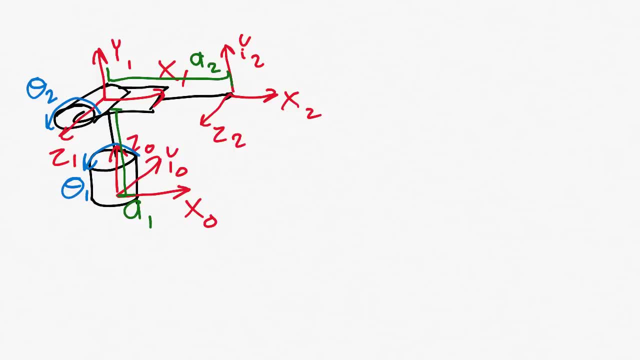 I've labeled the joint angles and I've labeled the link lengths And I've also assigned the frames according to our Denevet-Hartenberg rules. Let's use the Denevet-Hartenberg method to find the homogeneous transformation matrix. We're only going to do the second step right. 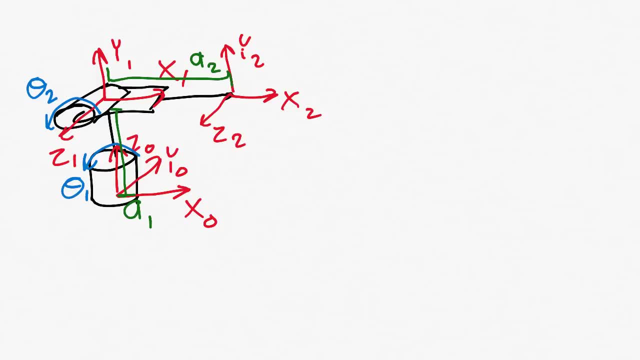 now find the parameter table, because I haven't yet shown you the third step. Let's find the parameter table. We know that our parameter table needs to have four columns because there are four parameters and we need one column for each parameter. There are two rotational parameters called theta. 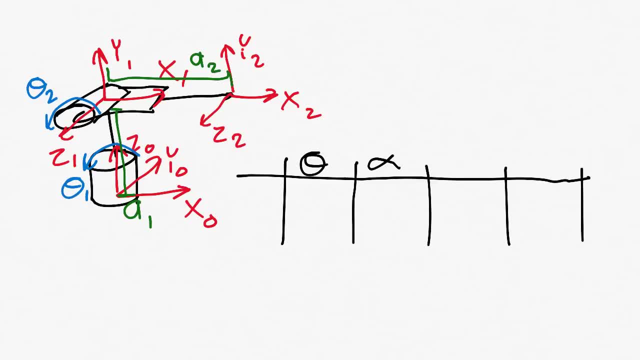 and alpha, And there are two linear parameters called r and d. We need to have a number of rows equal to the number of frames that we have, minus one. So I have three frames here and that means I need to have two rows. I'll call them row one and row two. Now, when I find the 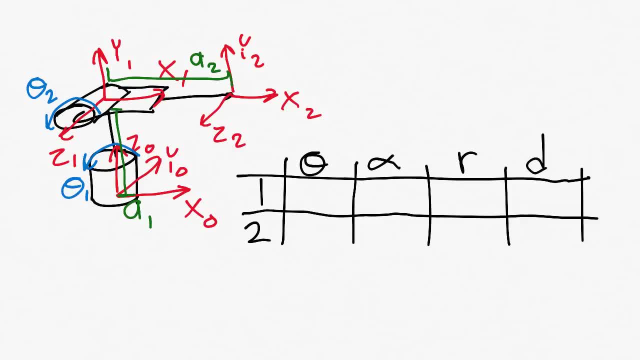 parameters. for the first row, I'm going to be looking at the relationship between frame zero and frame one. In other words, frame one is going to be my frame n and frame zero is going to be my frame n minus one. Theta is defined as the amount of rotation around z n minus one. between these, 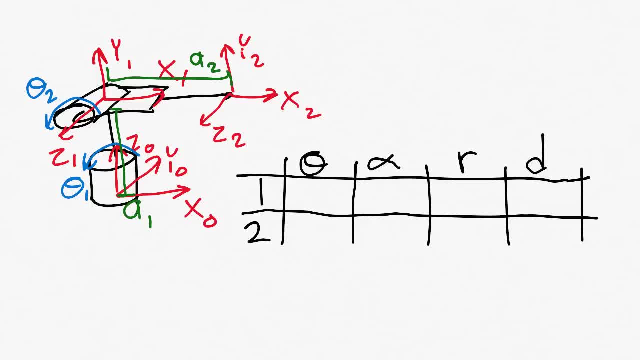 two frames: Z n minus. one in this row is z zero, So I have to write here the amount of rotation that we have around z zero. We have to include both any rotation that is due to the joint variable as well as any rotation that is required to get these two frames to match. When you're finding theta. 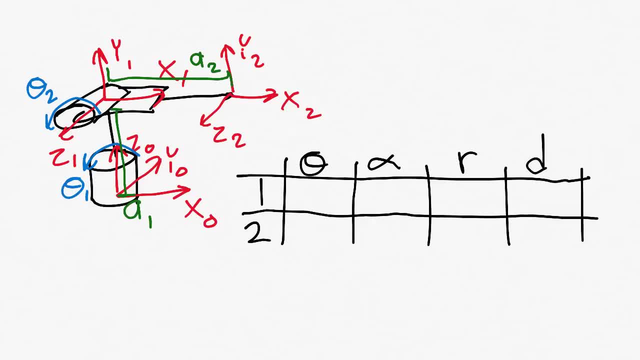 you want to pay attention mostly to the relationship between the two x-axes. In this case, my two x-axes are already pointing the same direction. That means that the only rotation around z that we have here is theta one. Let's do theta for the second row right away also. 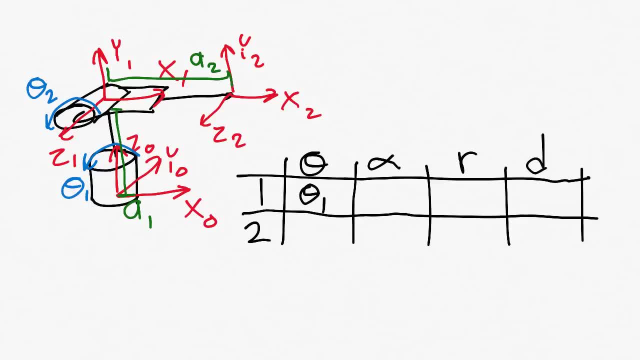 When we look at the second row, we're looking at the relationship between frames one and frame two. x one and x two are already in the same direction, So the only rotation that we have around z n minus one, that is, z one, is theta two. 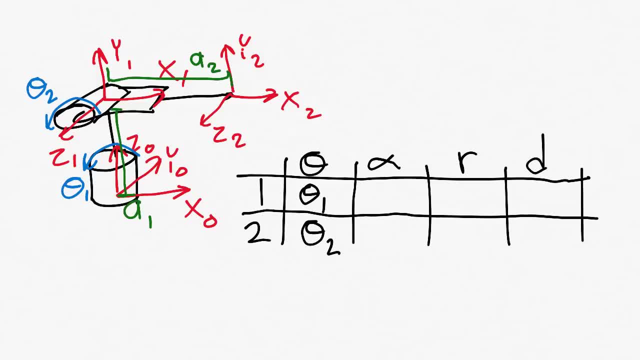 So I'll write theta two here. Now let's move on to alpha. Alpha is defined as the amount of rotation- rotation around xn- that is required to get the frame n-1 to match frame n. Let's look at the first row. 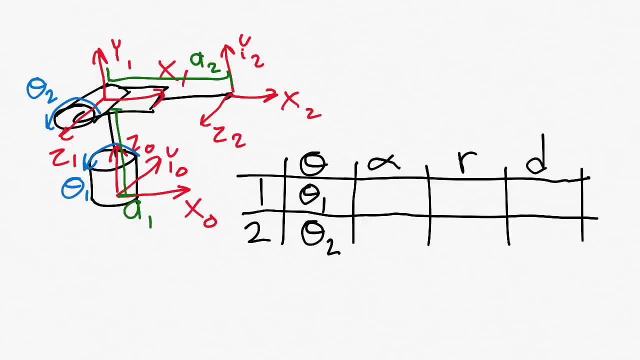 In the first row we're comparing frame 0 to frame 1.. We're going to ask ourselves: how do I have to rotate frame 0 around the axis x1 in order to get frame 0 to match frame 1.. We want to be paying attention mostly here to the relationship between the two x-axis. 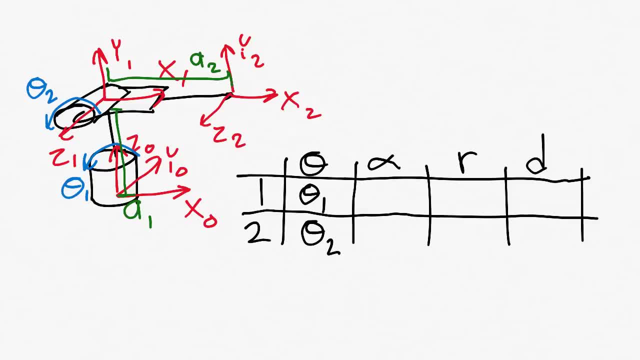 If I would rotate frame 0 around x1 90 degrees, z0 would come down and point out of the page which would match axis z1.. So the amount that I have to rotate frame 0 isена around the axis x1 is 90 degrees. Let's do alpha for the second row right away. 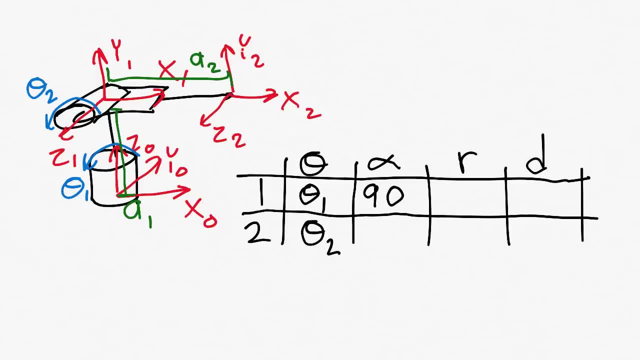 also In the second row, we're comparing frame 1 to frame 2.. I want to ask myself how do I have to rotate frame one around the axis x2 in order to get frame 1 to match frame two? And I can most easily tell this by looking at the relationship. 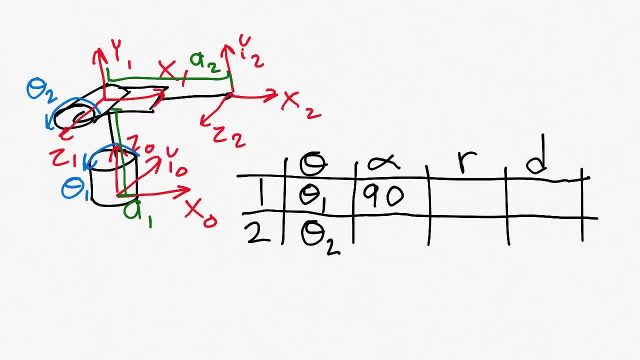 between the two z-axes, Since the two z-axes are already pointing in the same direction. that tells me that I don't have to rotate frame one around x2 at all order to get frame 1 to match frame 2.. So alpha here is 0.. Next let's do the 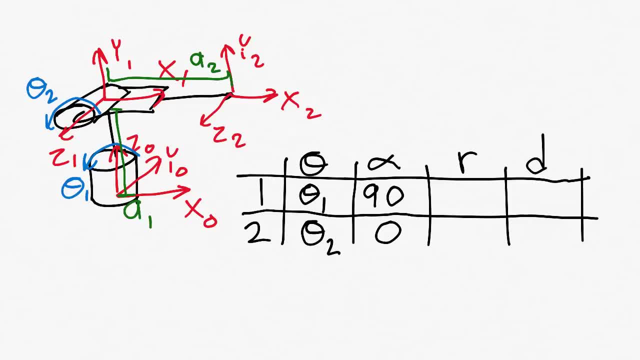 parameter r. r is defined as the displacement along x n between the centers of the two frames. In the first row we'll compare frame 0 to frame 1.. We want to ask ourselves what is the displacement between the center of frame 0 and the center of frame 1 in the x n- in this case x 1, direction, Here the? 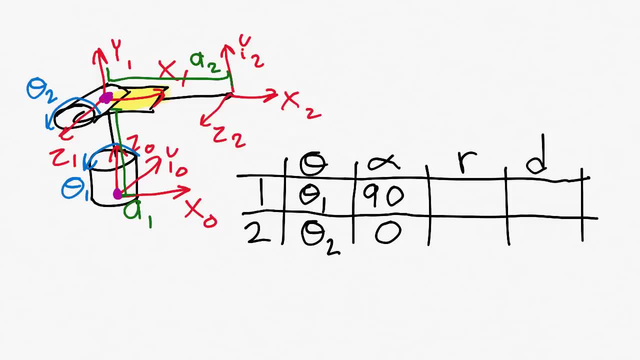 centers of frame 0 and frame 1 do not have any displacement in the x 1 direction, and so r in this row of the parameter table is 0.. Next let's look at the second row. In the second row we're looking at the difference between the center of frame 1 and the center of 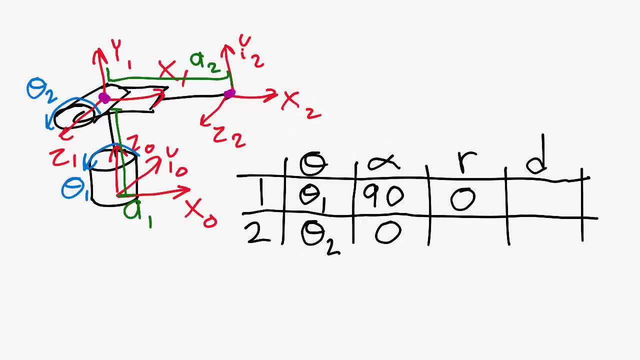 frame 2.. How far apart are these two centers? r is defined as the distance between these centers in the x? n direction, which here is the distance between the centers in the x? n direction and the center of frame 1 and frame 2.. Here is x 2.. How far apart are these two centers in? 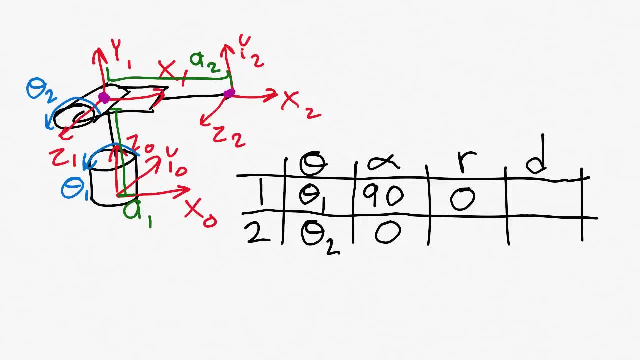 the x 2 direction. Here the distance is a 2.. Previously, when we found the displacement vector and the rotation matrix separately, we had to be very careful to think about whether our answer would be correct, no matter what the value of theta 2 would be. 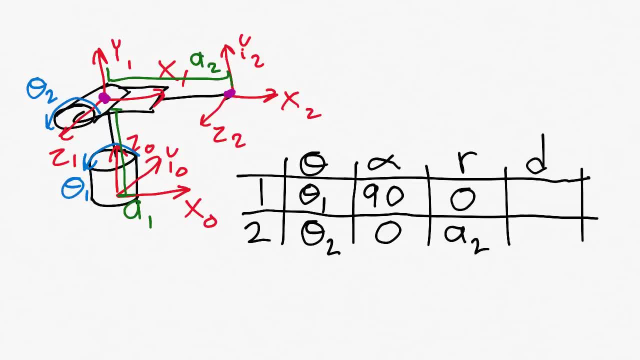 In the Deneveit-Hartenberg method. this effect is taken care of for us after we plug in these numbers into the matrix in the next step. So here all we have to do is think about how it is right now in the diagram Along the x 2 direction, the 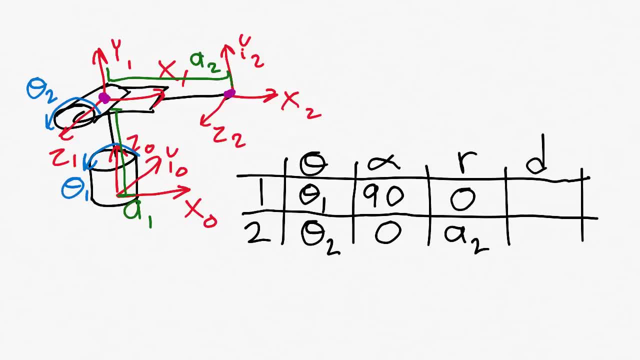 distance between the centers of these frames is just a 2.. Let's move on to the d parameter. d is defined as the distance between the centers of the two frames in the z direction. Let's do the first row Here. we want to. 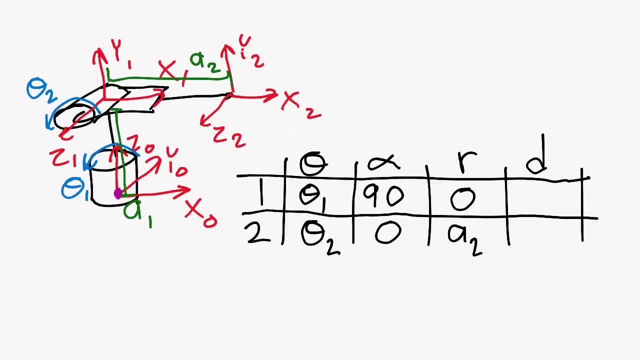 think: what is the distance between the center of frame 0 and the center of frame 1 in the z? in this case the z direction Here that distance is is a1, so I'll fill in a1 in the parameter table. Let's do d for the second row. 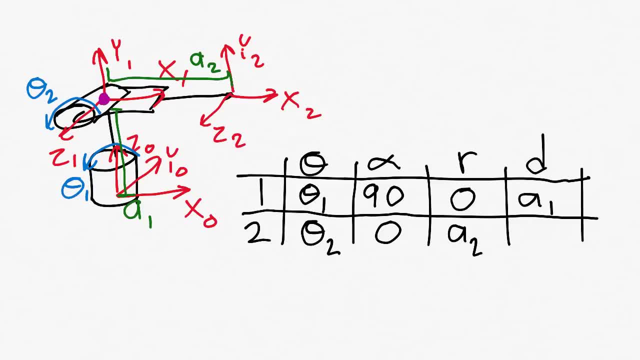 Here I want to think: what is the distance between the center of frame 1 and the center of frame 2 in the zn minus 1 direction, which here is z1? In the z1 direction, these two centers of the frames? 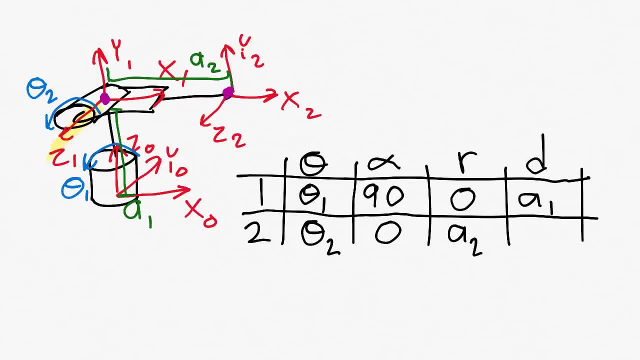 are lined up exactly. So d2,- that is, d in the second row, is 0.. I've now finished filling out my parameter table. Before I show you the second step in the Denevet-Hartenberg method, I want to show you a couple more examples of finding. 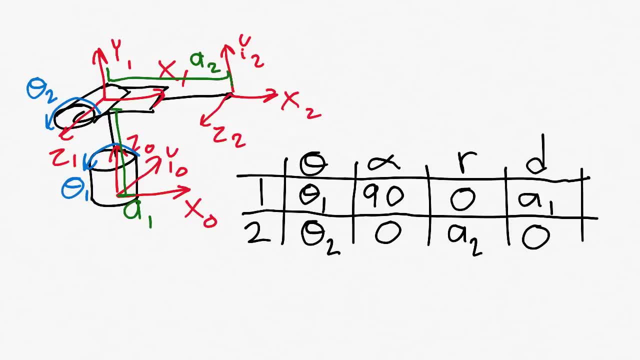 this parameter table. Becoming good at finding the values in the parameter table simply takes some practice. So let's do a little bit of practice. now I'm going to show you another kinematic diagram, If you think you've caught on to how. 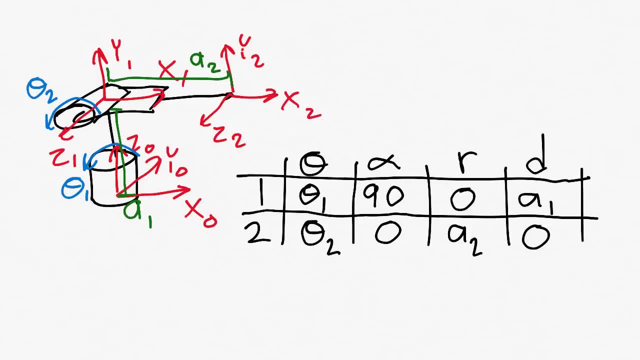 we fill in the values of the parameter table. pause the video after I've shown you the kinematic diagram and see if you can find the values of the parameter table on your own, And then resume the video and check your answer against mine to see if you got it right. 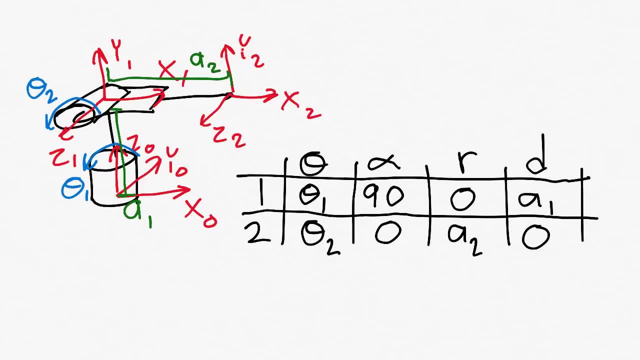 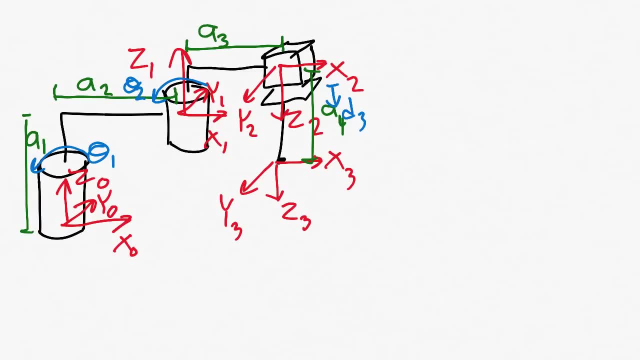 If you're still feeling pretty unsure about how we find these values, just watch This. let's me show you anotherowers example that you may want to watch the video and see if you can catch on after the next example. Here I'm showing the kinematic diagram. 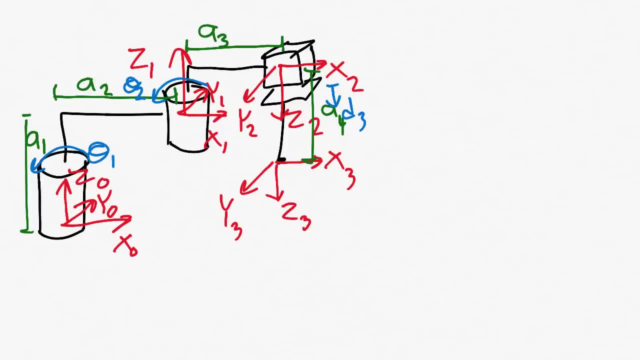 for this skeram manipulator. So we know that our parameter table is going to have four columns, because we always need to have one column for each parameter. We also need to have one fewer rows than the number of frames. I need to have three rows. Let's call them row 1, row 2, and row 3.. I'm going to 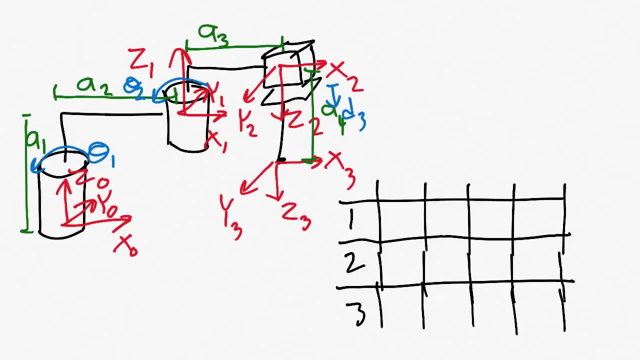 label the columns for the four parameters: theta, alpha, R and D. It doesn't matter what order you put these parameters in, you just have to include all four of them. Let's start with theta. Theta 1 is found by comparing frame 0 to frame 1.. 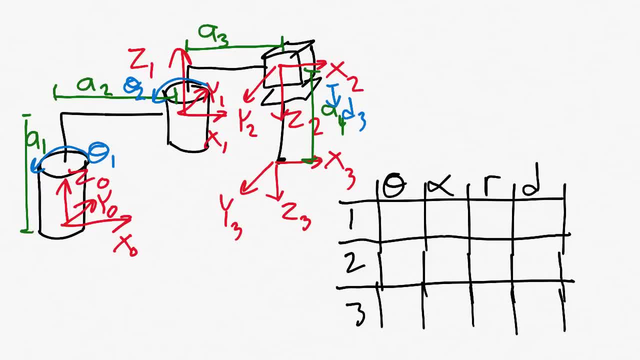 Theta is defined as the amount of rotation that we have around z n minus 1.. In this case, that is z 0.. We have theta 1 as being part of the rotation around z 0.. We also have to check to see if we have any additional rotation around z 0. that. 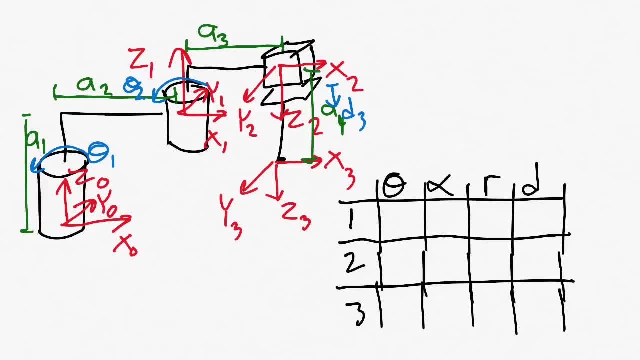 is needed to get x 0 to match x 1.. Since x 0 and x 1 are in the same direction, the only rotation we have here for theta 1 is theta 1.. Let's look at theta for the second row. Here we're going to compare frame 1 to frame 2.. 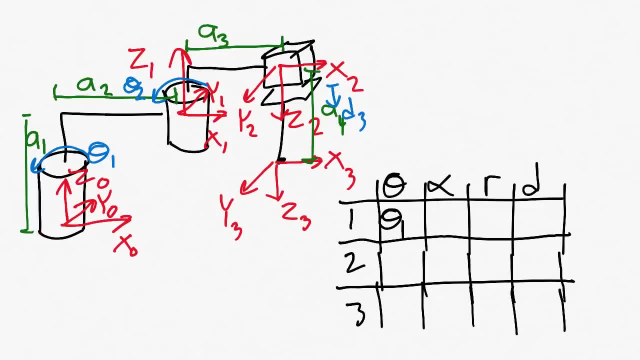 To see if theta can be rotated a little from table 2. we've got, say z n minus 1 around z 0, to 2 x-axis. We should change that to theta 2 and start with theta 2.. There's also theta 1, here an initially oscillating equation. 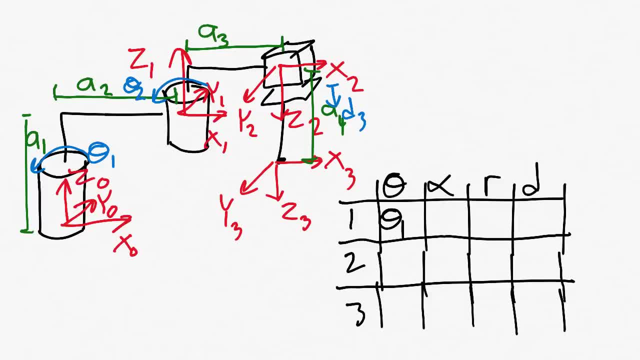 Now, this is theta 1, is this an oscillating equation? Well, in this example, we do have a rotation around z n minus 1.. Now let's look at our common variation. Theta 2 is the rotation around z n minus 1.. We actually just have to take care of that. to look for the x-axis, which is in the same direction, part of the rotation that we have for theta here is theta 2.. That's a rotation around z, n minus 1.. In this case, n minus 1 is frame 1.. 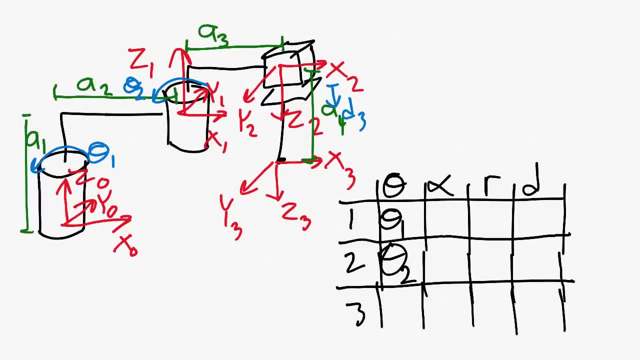 Next we have to look to see if the 2 x-axis are in the same direction. Here x 1 and x2 are in the same direction, theta 2.. Let's look at theta for row 3.. Here we're going to be comparing frame 2 to frame 3.. 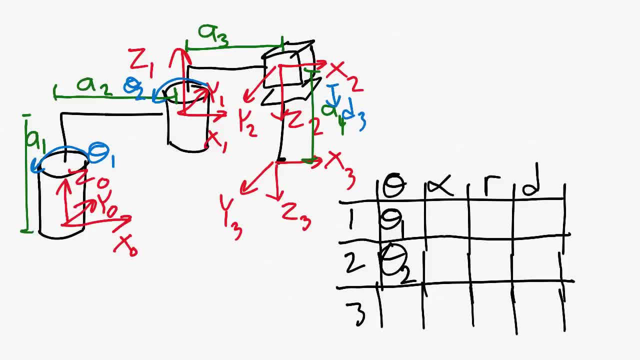 How much rotation do we have around Z2, between these two frames? Well, x2 and x3 are in the same direction, so we don't have any rotation due to that. But also we have no rotation due to the joint, because this is a prismatic joint. 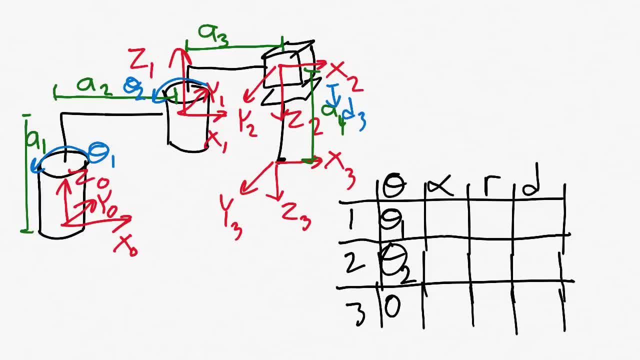 So theta for row 3 is 0.. Let's look at alpha. Alpha is the rotation around xn that we need to get frame n-1 to match frame 1, or n-1 to match frame n. In the first row we're going to compare frame 0 to frame 1.. 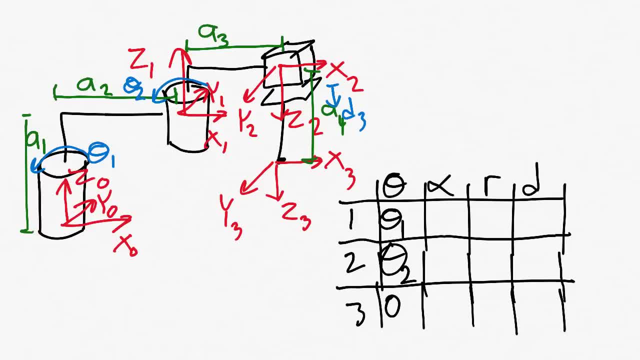 We're going to ask ourselves: how do we have to rotate frame 0 around the axis x1 to get frame 0 to match frame 1.. Since these two frames are already oriented exactly the same, we have 0 for alpha here. Let's do alpha for the second row now. 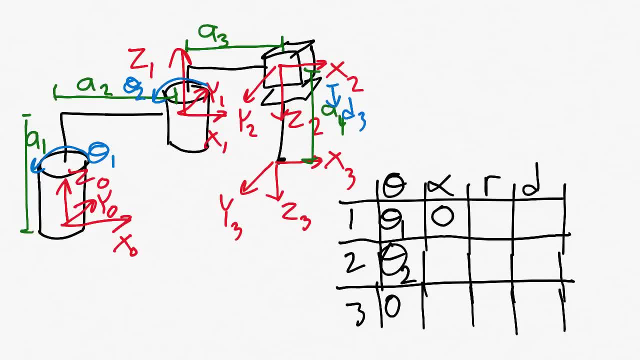 We're going to compare frame 1 to frame 2.. We're going to ask ourselves how do we have to rotate frame 1 around the axis x2 in order to get frame 1 to match frame 2.. Specifically, we're going to pay attention to the difference in the directions between: 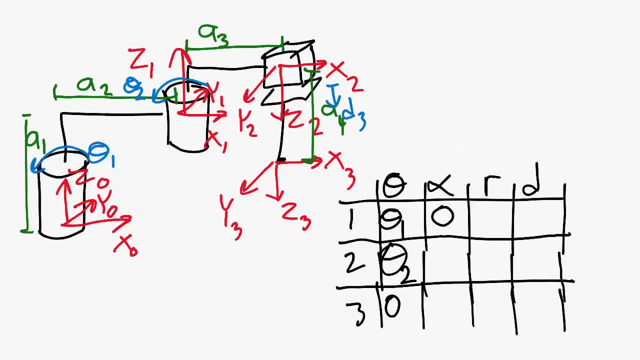 the Z axes. Since Z1 is pointing up and Z2 is pointing down, we would have to rotate frame 1 one-hundred and eighty degrees around the direction x2 in order to get Z1 to be matching frame 2.. So alpha in row 2 is 180.. 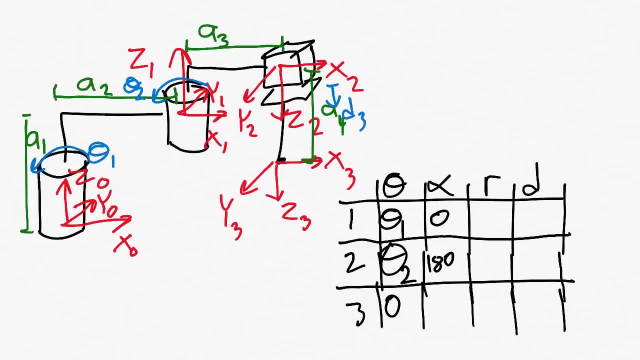 Let's try and find alpha for row 3.. Here we're going to ask ourselves how do we have to rotate frame 2 around the axis x3 in order to get frame 2 to match frame 1.. We're going to ask ourselves how do we have to rotate frame 2 around the axis x2 in order? 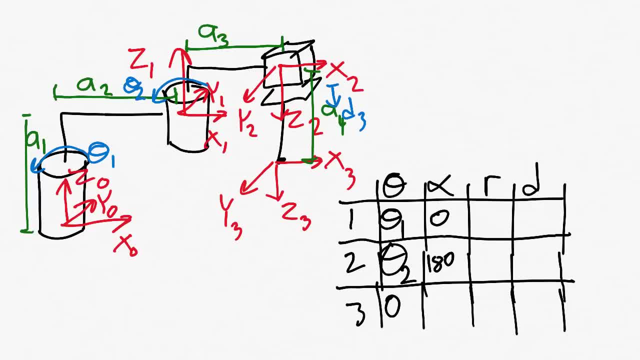 to get frame 2 to match frame 3.. And specifically, we'll pay attention to the directions of the Z axes. Since Z2 and Z3 already match, we don't need to rotate frame 2 around x3 at all in order to get it to match. 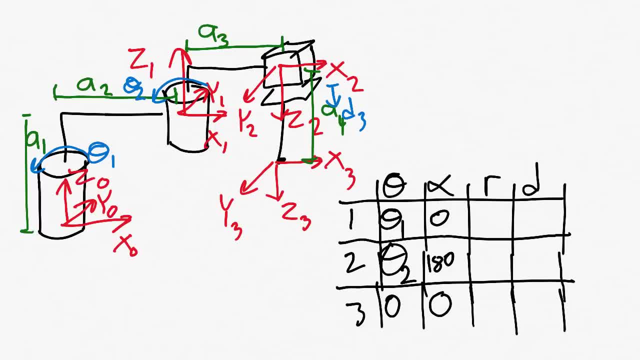 So alpha for row 3 is 0.. Let's look at R. R is the displacement between the two frames. In the first row we have x1 and x2.. We're going to ask ourselves how do we have to rotate frame 2 around x3 in order to get? 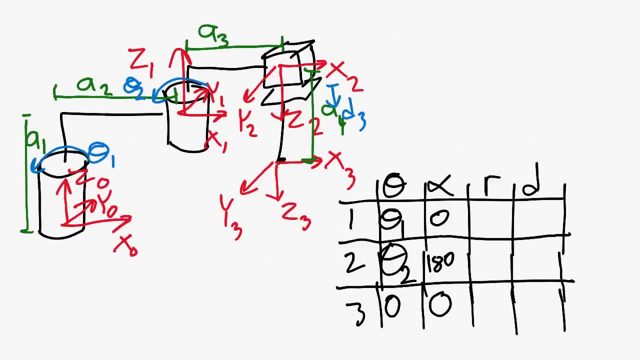 R to match The xn direction. So for row 1, we're going to look at the distance between the center of frame 0 and the center of frame 1, specifically in the x1 direction. The distance between these two frames in the x1 direction is a2.. 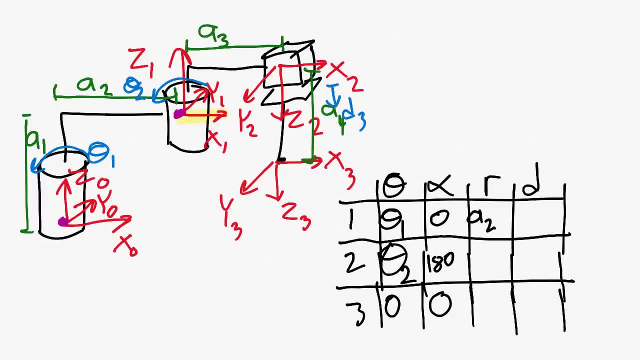 So R in the first row is a2.. Let's look at R for the second row. Here we are going to look at the distance between the center of frame 1 and the center of frame 2 in the x2 direction. The distance between the center of frame 1 and the center of frame 2 in the x2 direction. 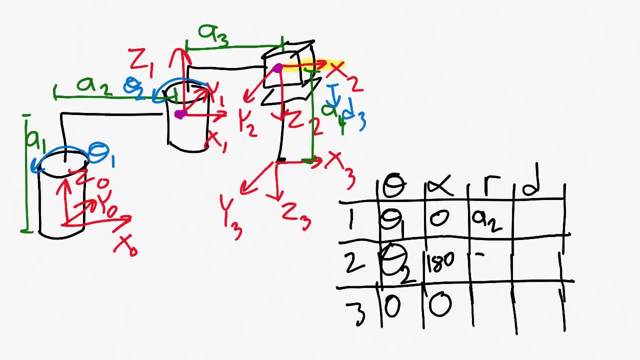 is a3.. Okay, let's try to get R for the third row. Here we are going to look at the distance between the center of frame 2 and the center of frame 3 in the x3 direction. The center of frame 2 and the center of frame 3 is exactly lined up in the x3 direction. 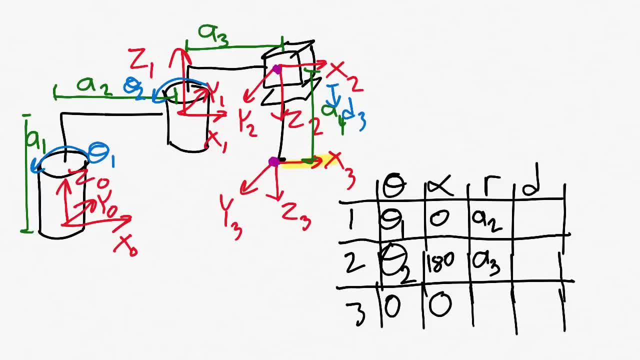 So R here in the third row is 0.. Lastly, let's fill in the D column. D is defined as the distance between the centers of the two frames in the z direction. So for the first row we are going to look at the distance. 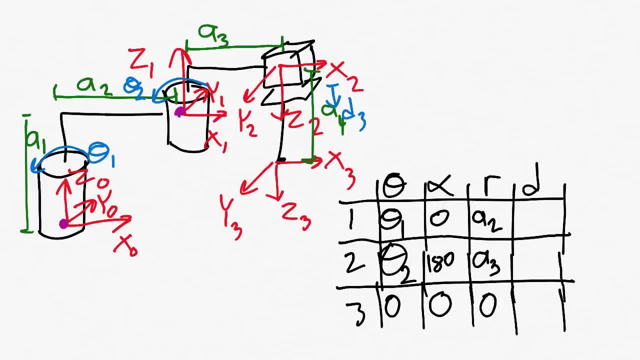 between the center of frame 2 and the center of frame 3 in the x3 direction, The distance between the center of frame 0 and the center of frame 1 in the z0 direction. Here that amount is a1.. Now let's look at the second row. 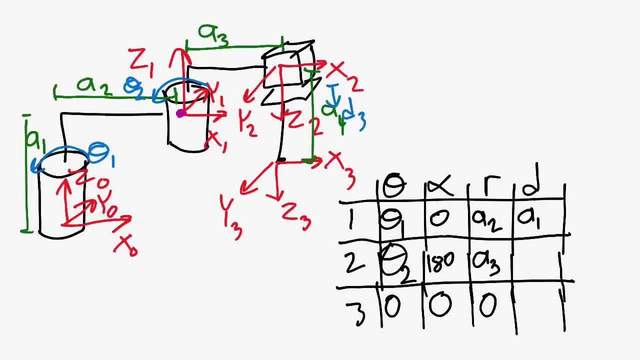 Here we are looking at the distance between the center of frame 1 and the center of frame 2 in the z1 direction. When I try to write this amount into my table, I notice that I forgot to label one of the link lengths. I have a link length here that I didn't label. 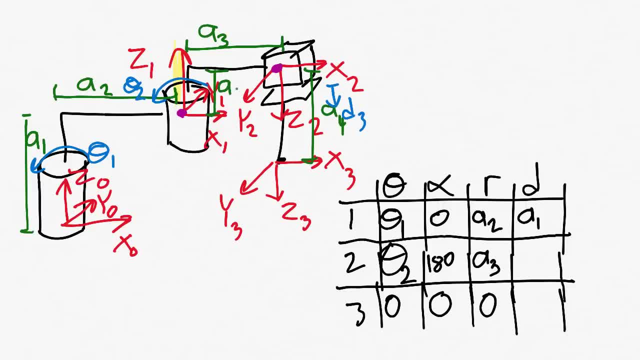 I'm going to fill it in now and call it a5.. So D for row 2 is a5.. Lastly, let's do D for the third row. Here we are going to look for the distance between frame 2 and frame 3 in the zn-1 direction. 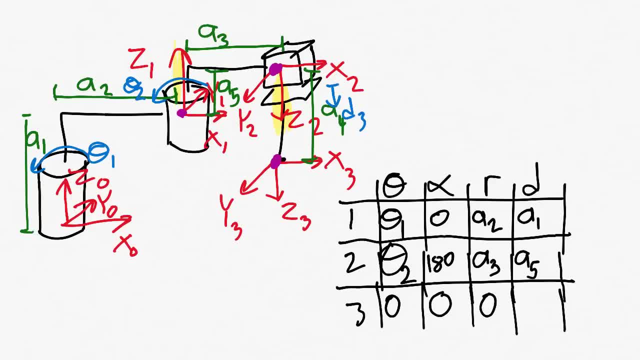 which here is the z2 direction. The distance here is a little bit tricky because we have both a link length and also a joint variable. The distance here is a4 plus D3.. You might be wondering why I made a link length variable. It's because I want to know the distance between the center of frame 2 and the center of frame 3.. It's little trickier to measure that, estimate an angle, and then on your ZLIKEL經 huis어�ities, we will be able topg this as this series. 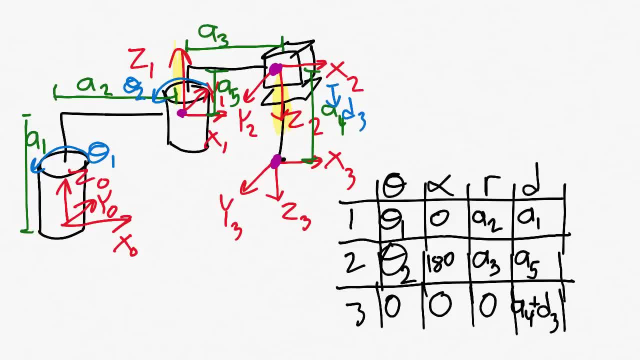 Just like I am always wondering why I made a4 plus D3 positive, even though they are pointing down the flip mark length appear. Note that in each of these parameters we are looking in a specific direction. In this case is D in the third row. we are looking at the z2 direction. 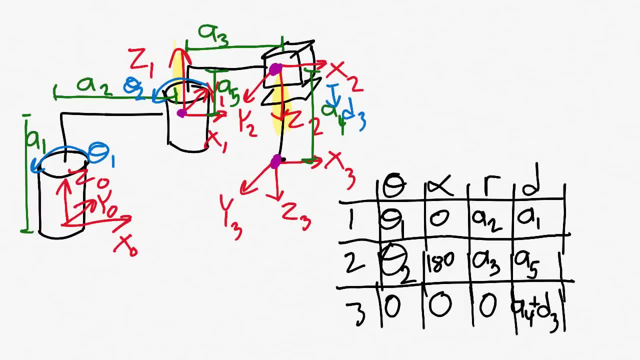 Z direction is positive in the z2 direction down, as indicated by our Z2 arrow. I am glad to let you know that there is ausan on z3 now. The z2 meaning is down now But it needs to have a方 slash D2 investors because Z2 is positive. 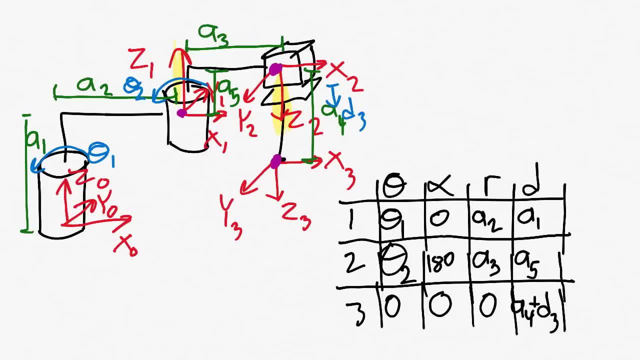 The random ş is positive and the z2ต is negative, So it is going to be positive. positive in this row of the table. If I had instead defined z2 to be up, which would be allowable in our Denevitt-Hartenberg rules, in that case I would have had to make a4 and d3 both negative. 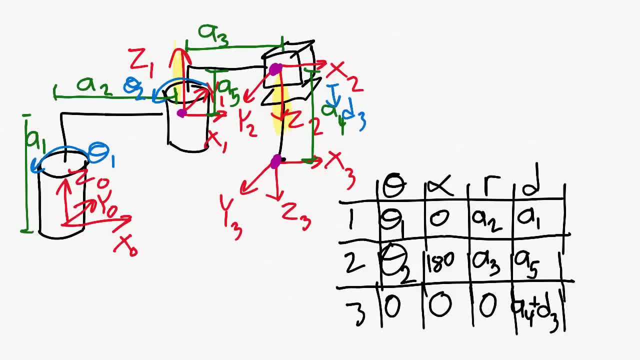 Now, as you do this method for more and more complex manipulators, it's a good idea to have some ways to check yourself for errors as you go along. One of the ways to do this is, once you have this parameter table filled out, you should have in your table every one of your joint variables and every one of your link lengths. 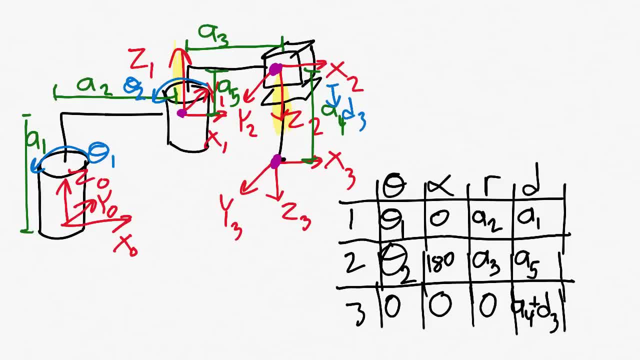 appearing somewhere. If I had filled out this table and would see that, for example, theta2 did not show up in my table, that would be a clue to me that I'd done something wrong, Since the joint motion theta2 actually does affect the rotation and position of the end effector. it needs to. 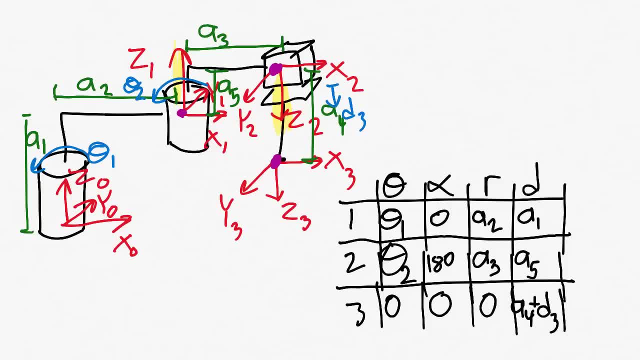 show up in my table somewhere. Similarly, if I would have filled out this table and found that say a4 did not show up, I would know that I had done something wrong, since the distance a4 really does affect the position and or. 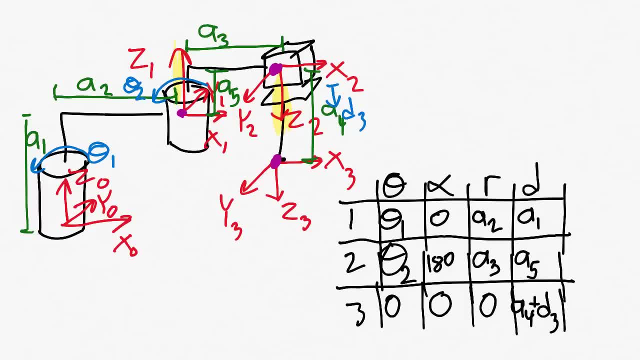 rotation of the end effector. I will be showing you some more complete examples in the next video, but before we finish this video, I need to show you the second step of the Denevet-Hartenberg method, which is how we use this parameter table to get the homogeneous. 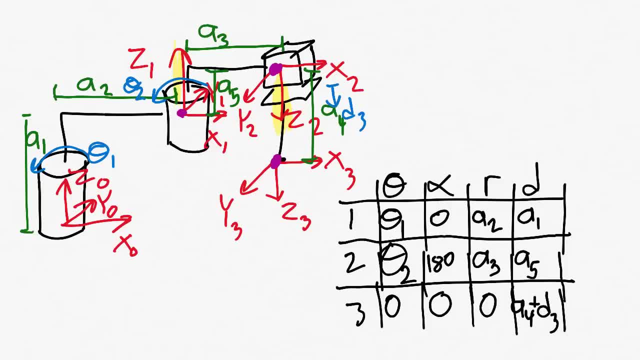 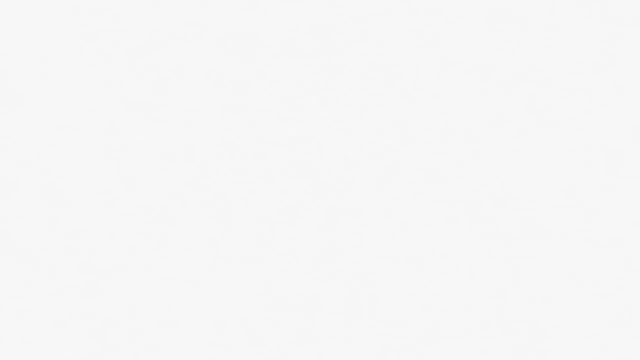 transformation matrix. It's actually a simple step. The hard step is finding this parameter table. If you've done this part correctly, finding the homogeneous transformation matrix is trivial. Once we've found our parameter table, we can find each homogeneous transformation matrix from frame n-1 to frame n by 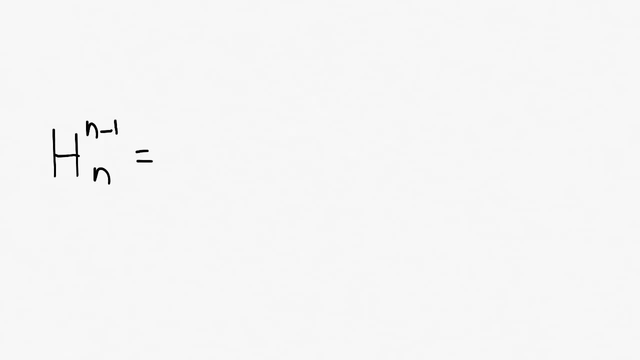 plugging in the parameters in each row of the table, one at a time, and we plug them in like this In this matrix I can plug. in my matrix I've used the letter c to represent the cosine and the letter s to represent 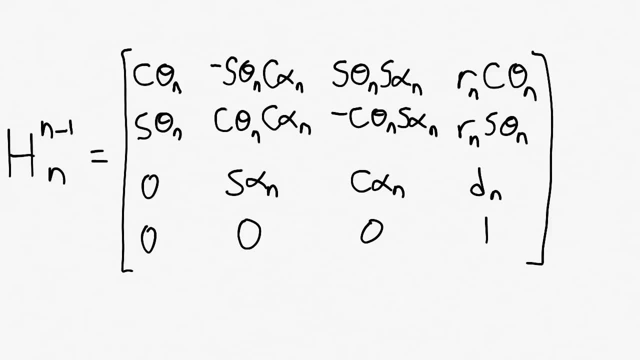 the sine. So suppose you want to find the homogeneous transformation matrix between frame 0 and frame 1, like this: 0 to 1.. In this case n is 1.. All we would have to do is plug in the four parameters that we found in row 1 of the table. Here n would be equal. 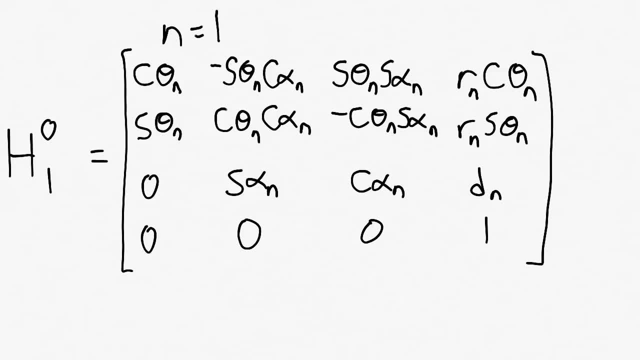 to 1.. Then let's suppose that we want to find the homogeneous transformation matrix from frame 1 to frame 2.. We can set n equal to 2, find all of the parameters from the second row of the table and plug them in. 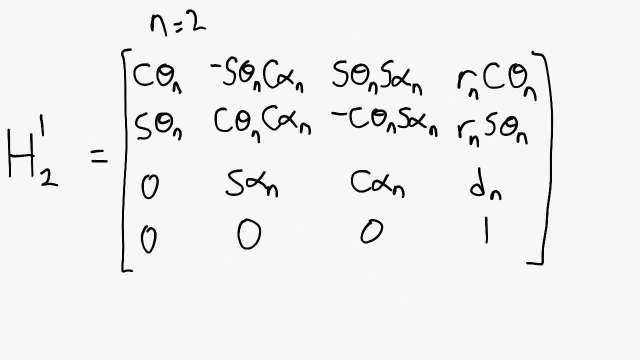 Then if we want to find the homogeneous transformation matrix from frame 1 to frame 3, or that is from frame 2 to frame 3, we set n equal to 3, plug in all of the parameters from the third row of the parameter table to find this matrix. Then we can find h from 0 to 3, all. 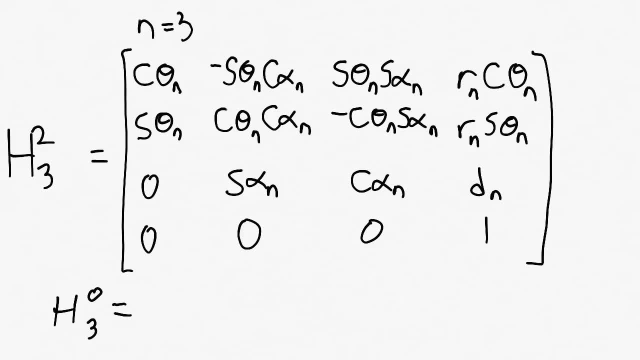 the way from the base frame to the base frame And this is what we get in the end effector frame by multiplying these three matrices that we found: h 0, 1 times h 1, 2 times h 2, 3.. Keep in mind that the meaning of the homogeneous